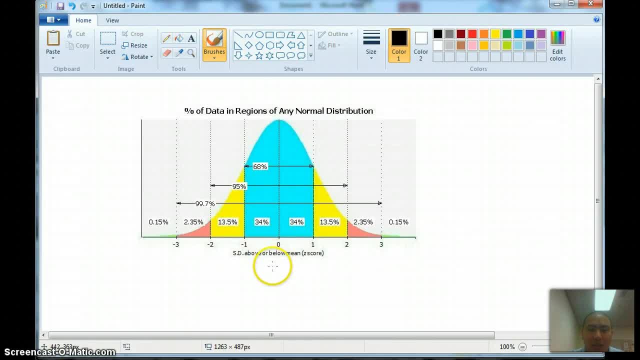 All right, you guys should have this already from our notes today And we said that the mean was 70. So that's 70. Over here would be 75. Then over here is 80. And I forgot a mouse today, so this is really hard for me. 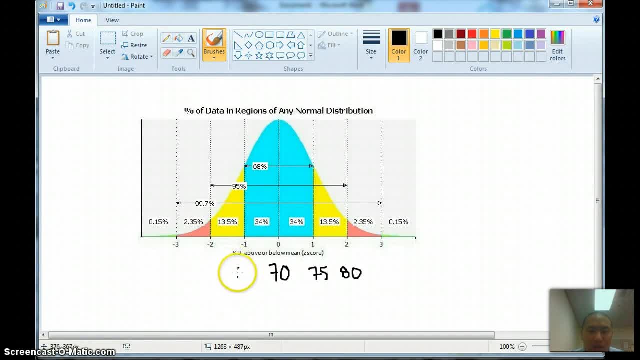 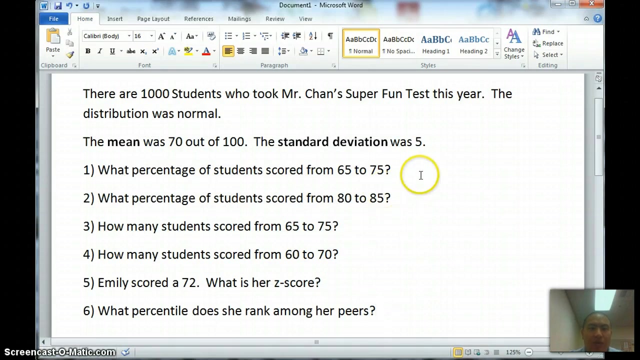 All right, and then I'm going to go the other way, which is 65,, 60, and 55. And I forgot, the other way is 85.. All right, so what the question is asking us is what percentage of students scored from 65 to 75?. 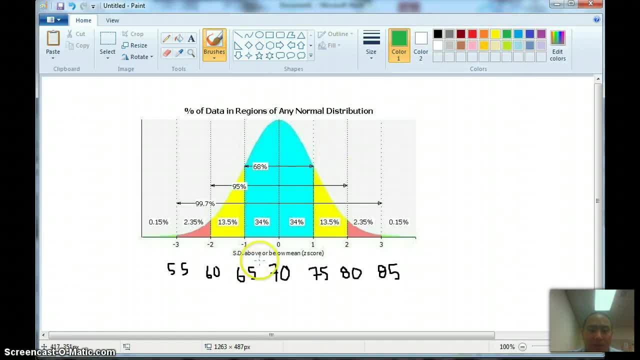 So 65 to 75.. So 65 to 75 would be from here to there. Okay, So from 65 to 75,. well, we're going to look at the percentage there. That's a total of 34 plus 34, and that's 68%. 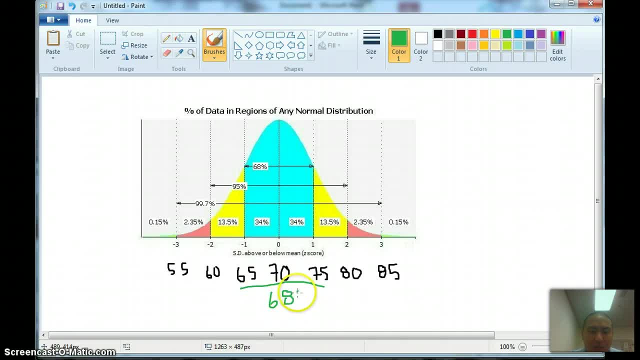 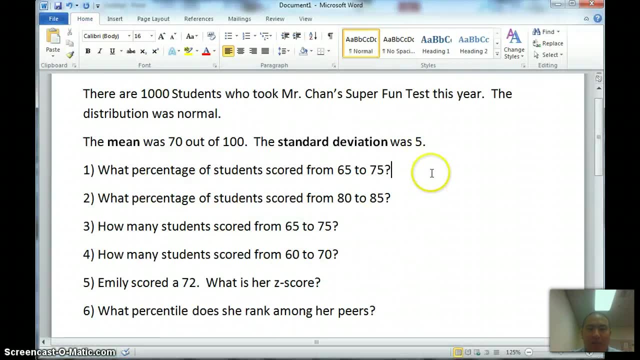 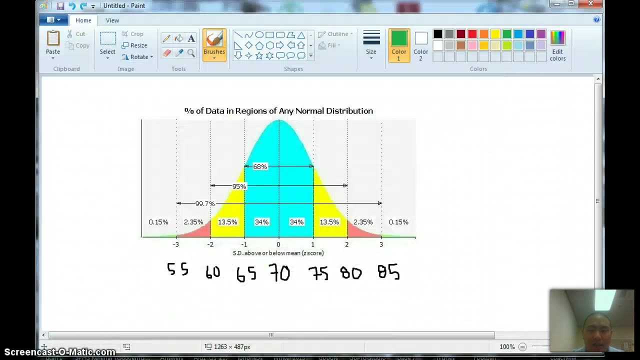 All right, so that's 68%. We know the answer for that one. All right, so let's go ahead and erase that off and write in 68%. All right, now the percentage of students that scored from 80 to 85, this one shouldn't be too bad either. 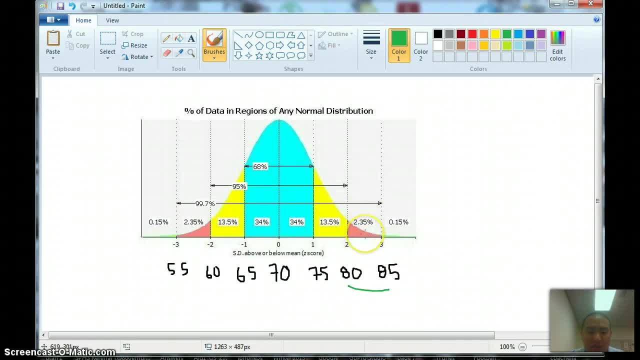 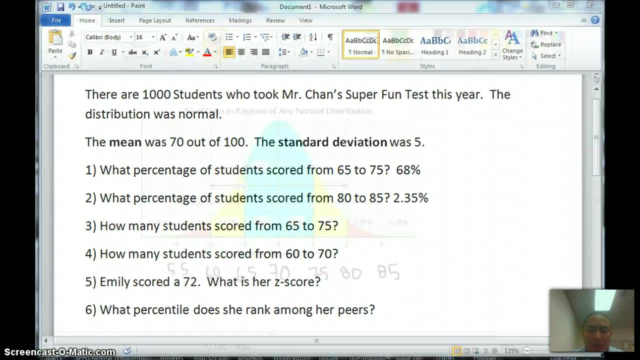 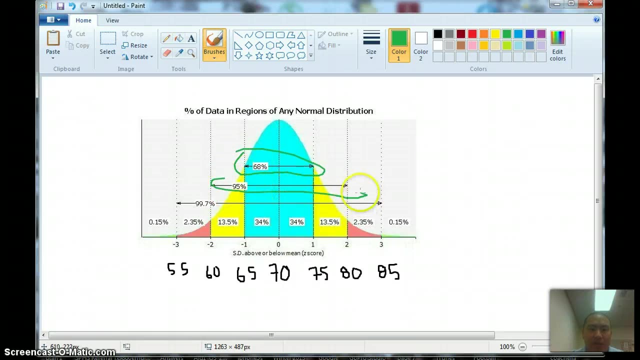 That's from here to here and that's 2.35%. Now, remember, all of this comes from the empirical rule and that's shown by this thing: the 68,, the 95, and the 99.7.. 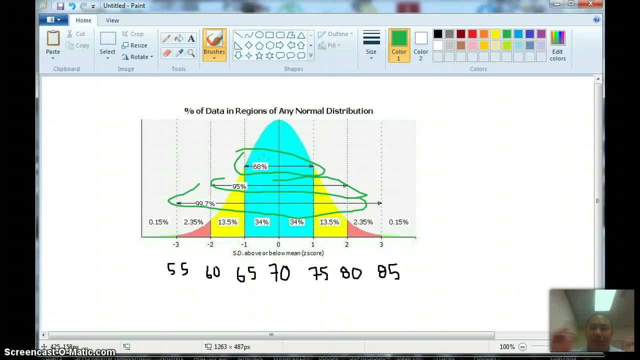 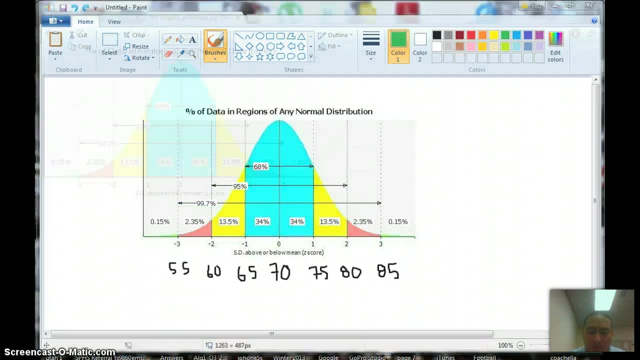 Okay, that's the empirical rule. If I go one standard deviation to left and right, I capture 68,, 295,, 399.7.. All right, so we've done the second question. Let's pull the third question up. 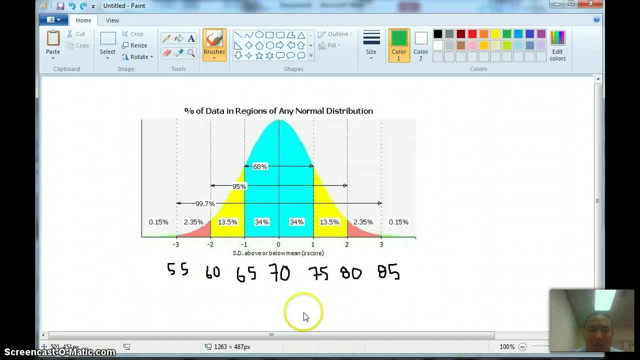 How many students scored from 65 to 75? So 65 to 75. Now, the difference between this question and the other one is that it says how many students. So we know that this is 68%, right, But it says how many students. 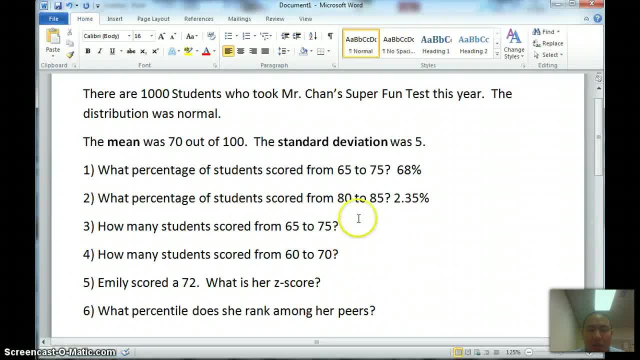 Well, now we have to go back to our original question, which is: there are 1,000 students. So if we want to figure out how many students, we know 68% of 1,000 students And in order to solve that, that would be the same thing as saying 0.68,. 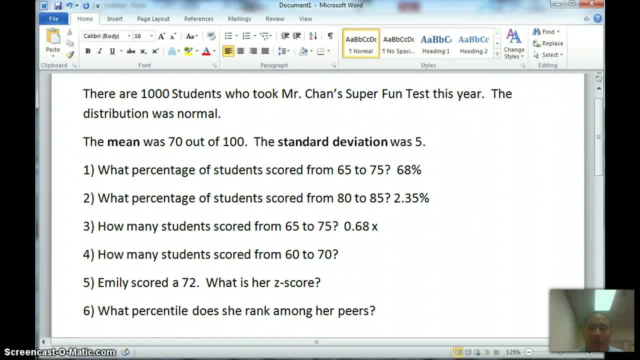 which is 68% as a decimal times 1,000.. And that should come out to be 680.. So 680 students scored between 65 and 75.. On my super fun test, All right, how many students scored from 60 to 70?? 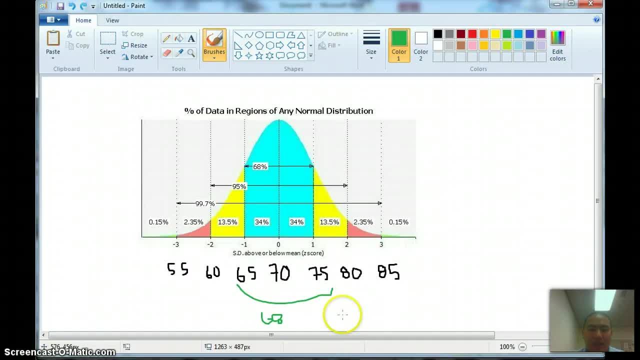 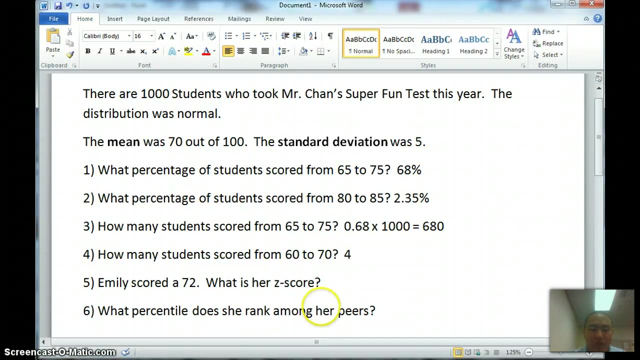 Now we need to look at this table again: From 60 to 70,, that looks like from here to here, And that is 13.5 plus 34%. That is 47.5%. So 47.5% of 1,000.. 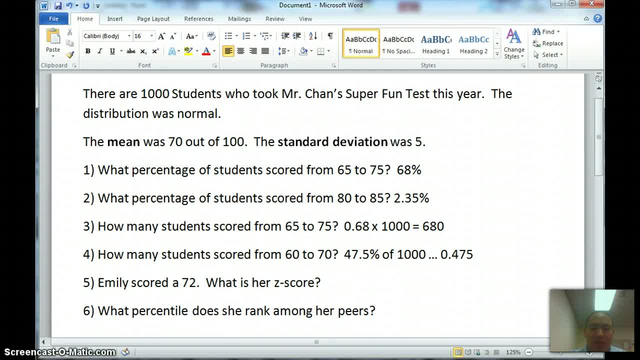 Well, we're going to write that out as 0.46.. So 475 times 1,000, and that gives me 475 people. So 475 people scored from 60 to 70.. All right, so now we're going to think about Emily. 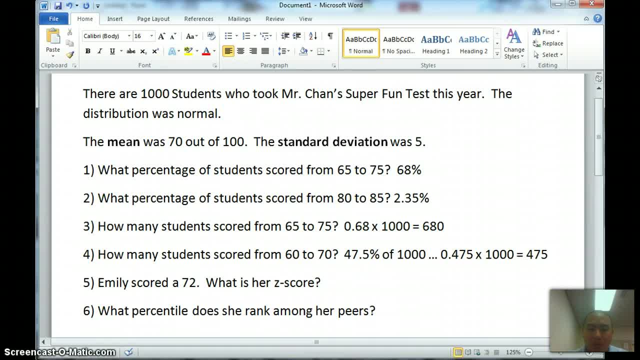 So Emily scored a 72, and we want to figure out what her z-score is. Now, remember the z-score. the formula is really not that important because you can just come up with the formula pretty easily. So I'll try to do this without the formula, and then we'll write it as a formula. 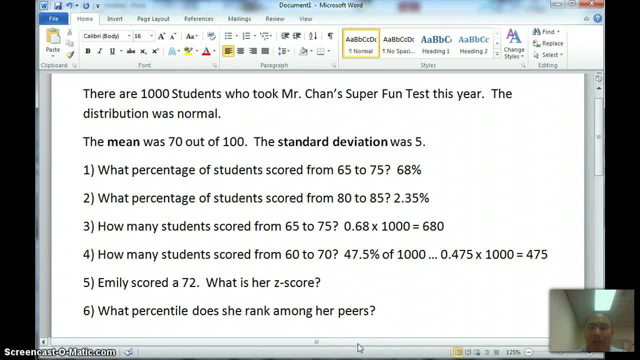 A z-score is the same thing as a standard deviation, Except now you're just looking at how far away to the right or how far away to the left you are, And now you have decimal values. So if Emily scored a 72, a 72 is somewhere over, like here, right? 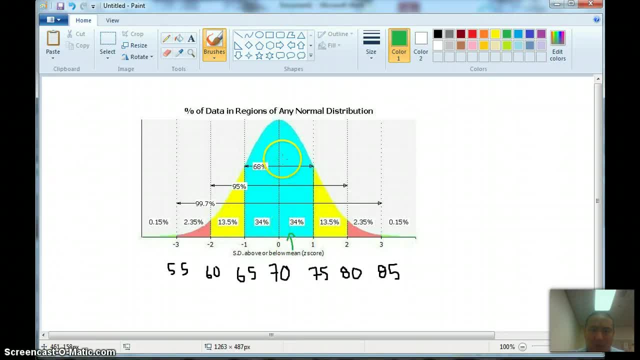 This is like 72.. Okay, now we want to figure out how many standard deviations away she is right And that would be our z-score. So this is our z-score, And I'll just put a little z here to know that that's our z-score. 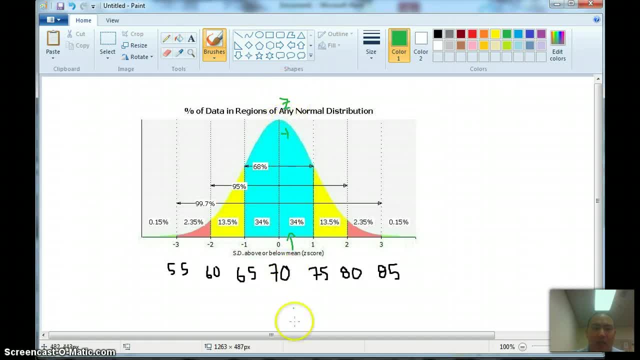 Okay, so we want to figure out how many standard deviations to the right. Okay, so to do that, we have this formula And essentially what it is. we need to figure out how much of a standard deviation is 72 compared to a standard deviation. 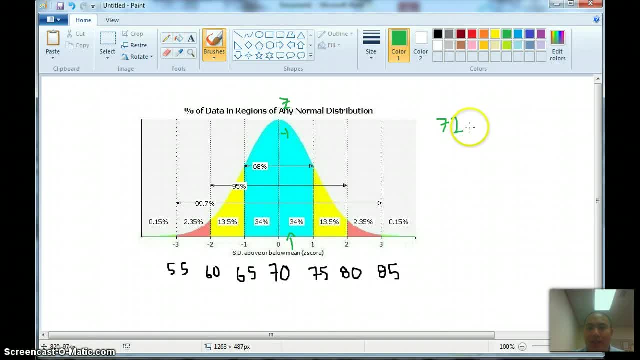 Well, if you have 72,, how far away is that from the mean? Well, that's only 2 away from the mean right, And that's 72 minus 70.. Now to figure what that is as a standard deviation, I just divide by standard deviation. 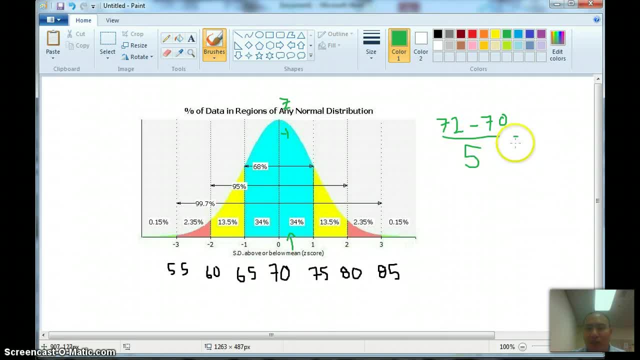 So the standard deviation. So in other words, I have 2 out of 5, right, I'm two-fifths of a standard deviation to the right, And what that is is 0.40.. And that's my z-score. 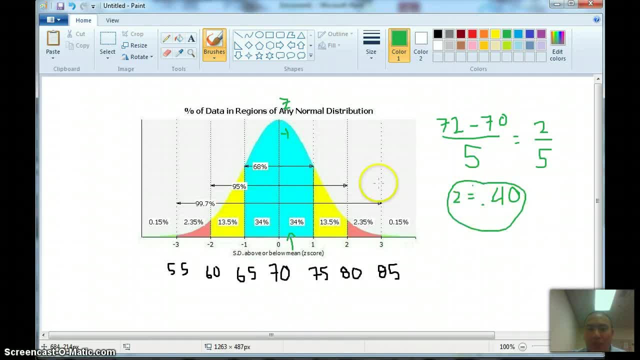 So all the z-score is: is this formula: what you have- and we wrote this down in class: what you have minus what the mean is divided by standard deviation, And that gives you a z-score And you could have a negative z-score and all that represents is that you're going to the left instead. 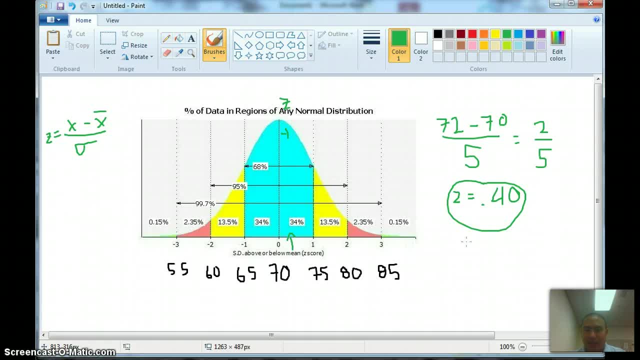 So we look at our z-score and it's 0.40.. And this is the part that's not included in our classwork today, And it might be included in the next lesson as well as our homework, And that would be this. 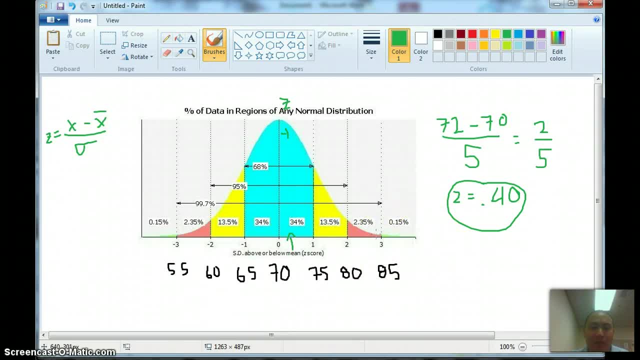 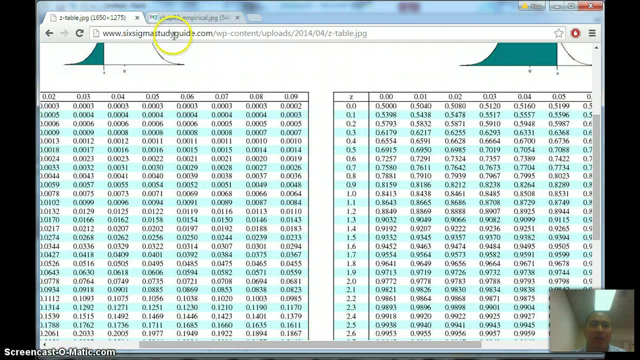 From the z-score, you can pull up what percentile rank you are. Okay, so, for example, let's go ahead and pull this up. Okay, I'm going to put this on our website And it's essentially a z-table, right. 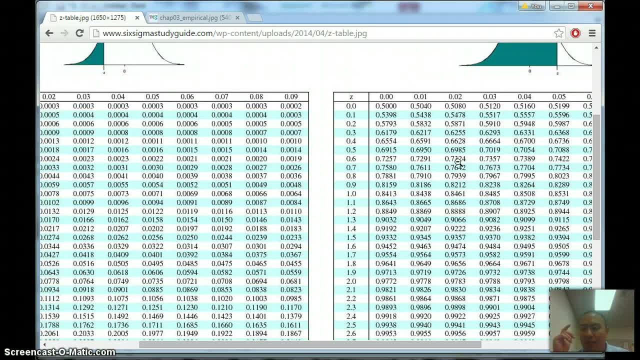 And this is the only way, outside of a computer or calculator, that you can figure out what percentile you are in. So remember, in class we said if you have a z-score of 0,, well then you're right at the mean, And that means you have 50% above, 50% below. 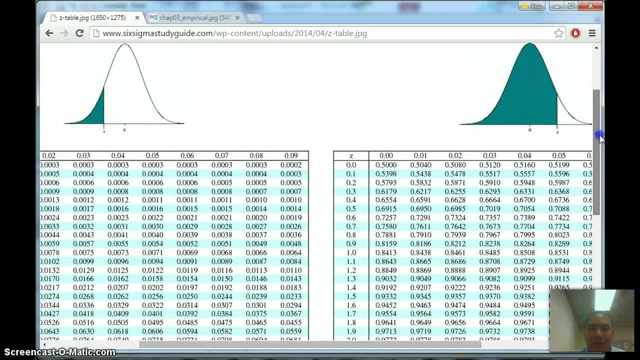 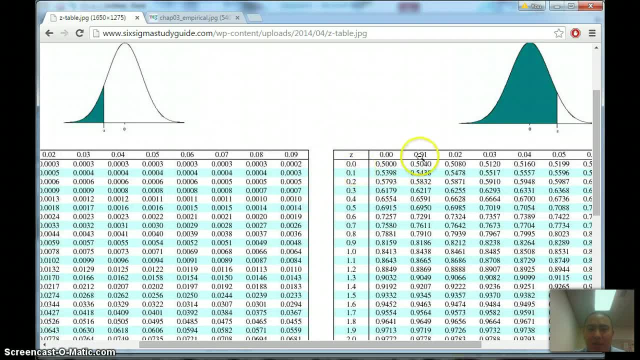 So what this z-score table does is it tells us what percentile rank we are. So if we're at z of 0, we're in the 50th percentile, If we're at 0.0.. And this part is the next part. 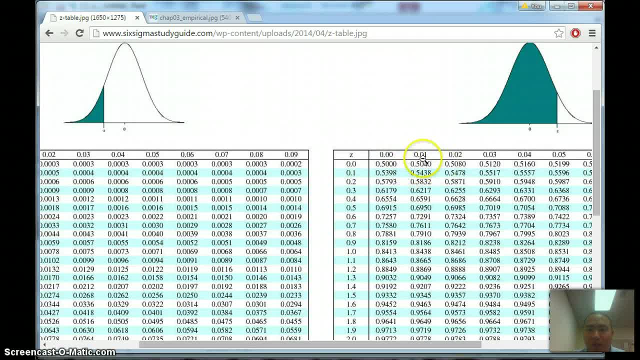 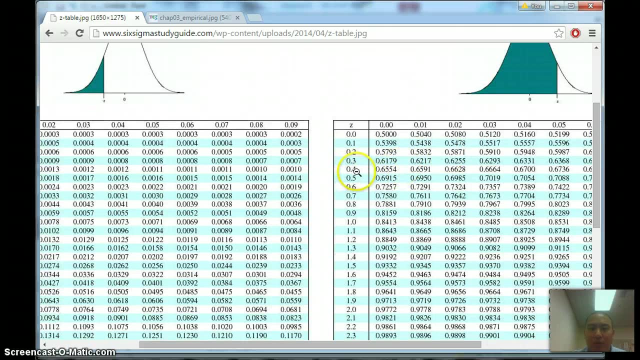 So it's 0.01.. Then we are at the 0.5040 percentile, In other words 50.4%. If we're at 0.02, we're at 0.5080.. Now we are looking for ourselves at 0.40, which would be right here.